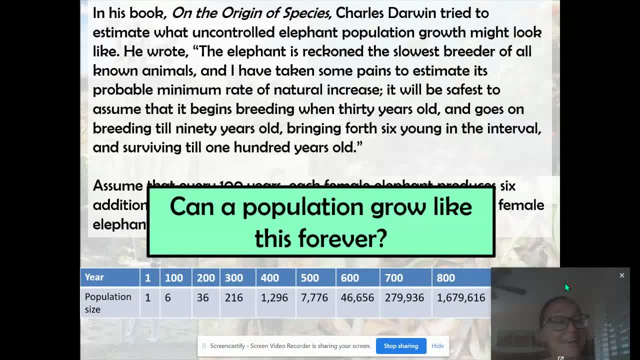 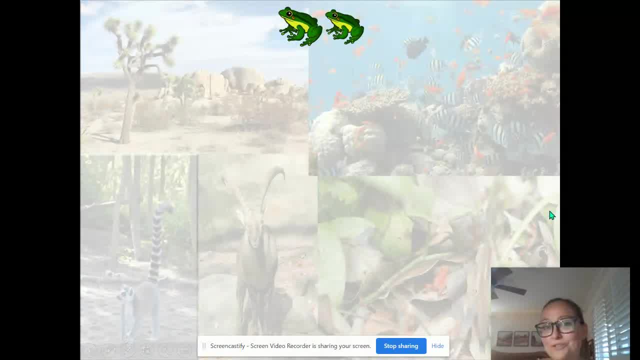 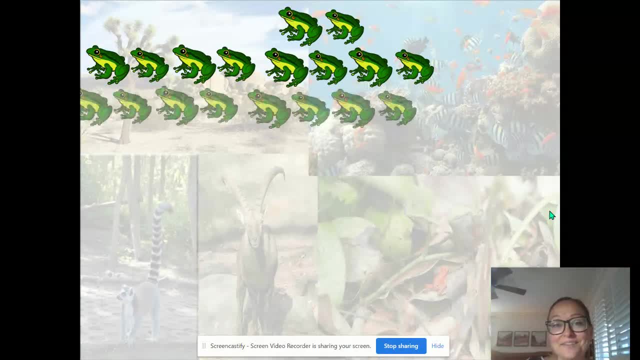 realistically, this growth could not go on forever like this right. So here we can look at it in a visual way: We have two frogs that reproduce and they have offspring, and now there's four, and then they reproduce, and now they double, and now there's eight, and then now we have 16.. And we just keep having. 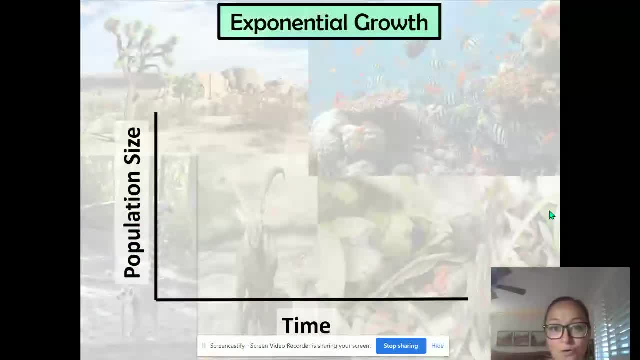 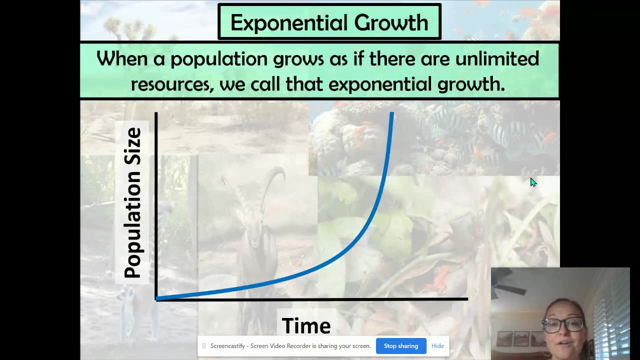 this exponential growth. If we were to graph this over time- whether it's the frog example or the elephant example- what we see is this J-shaped curve In exponential growth. the population grows as if there are unlimited resources. So exponential growth is often called a J-shaped or referenced. 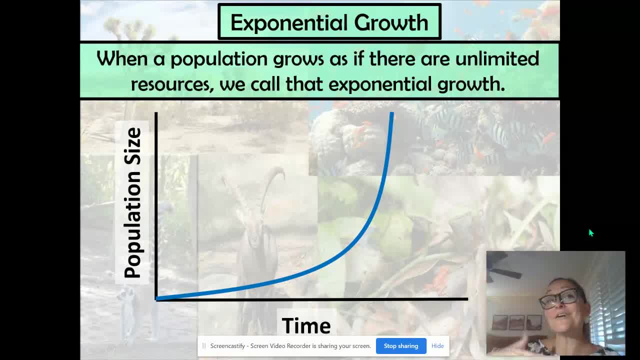 as a J-shaped curve and shows as if there was no like no bounds or no end to the possible resources for this population. And the population can grow indefinitely under exponential growth models. Now, sometimes populations really do grow exponentially, So if you have like a forest fire, for example, and the forest was all cleared, 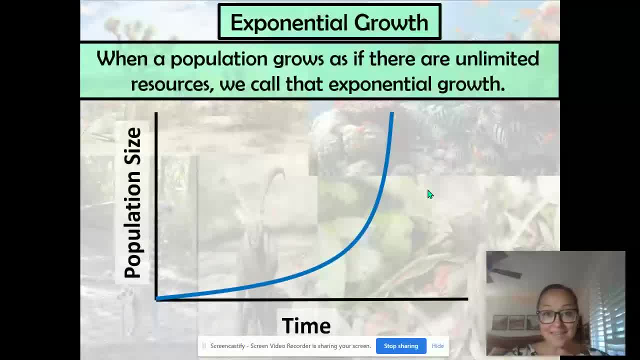 and then you have some seeds of new grassland that is going to experience exponential growth because it is a large-scale population. And so if you have a forest fire, for example, and you have, at least temporarily, as if there's- unlimited space, and unlimited sunshine And if it rains there's unlimited water, It would experience exponential growth. But realistically they can't grow forever. If we take that grass example following a forest fire, eventually it's gonna fill up. It'll run out of space, right? 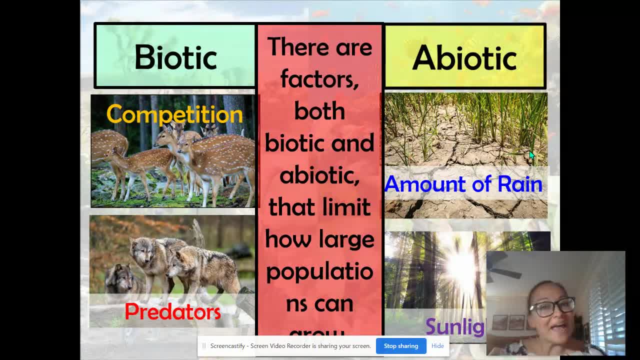 Or if the elephants, for example. they're gonna run out of food. We have these things called biotic and abiotic factors. They're gonna limit how large populations can grow. Eventually there'll be intense competition. Predators will start to have an impact on population size. You could have. abiotic factors like the amount of rainfall can limit how big a population grow or the amount of sunlight. If you're a tree growing in a forest, eventually trees growing on top of trees isn't gonna cut it. They'll cut off each other's sunlight supply. 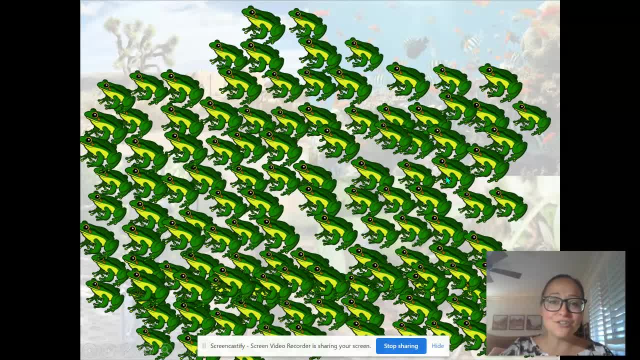 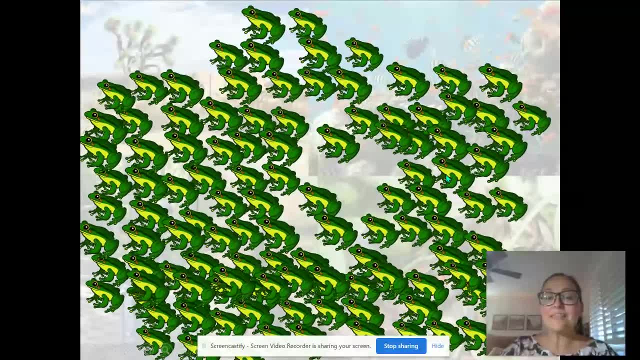 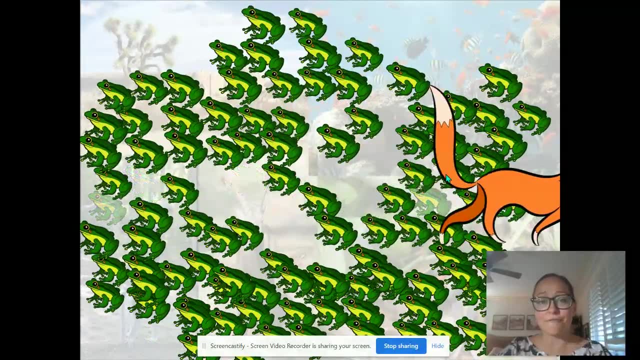 And so when we look at populations and why they generally can't grow exponentially and forever, it's because there's these things called limiting factors And they will limit how big a population can grow. So here I'm using the example of predators on these frogs. 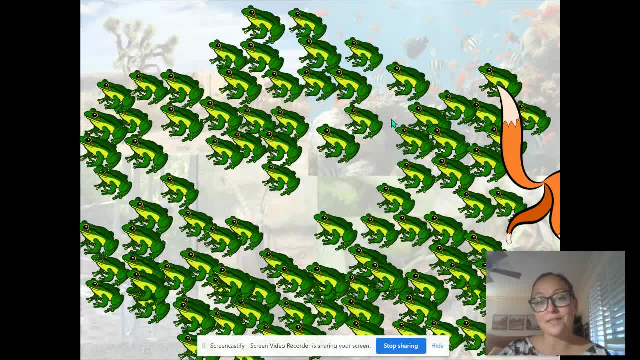 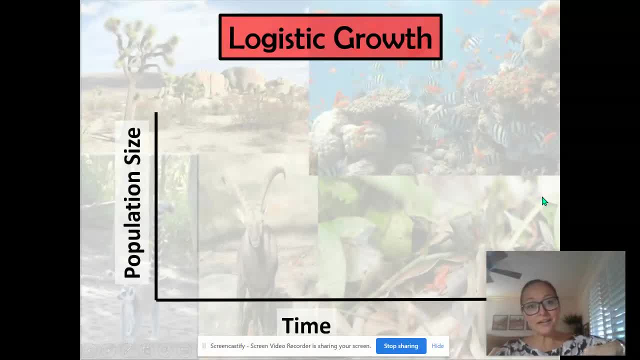 The foxes are eating the frogs and limiting how big that population grows. So when we look at logistically what happens in populations, they may experience initially a J-shaped curve, but eventually competition predators. they may experience initially a J-shaped curve. 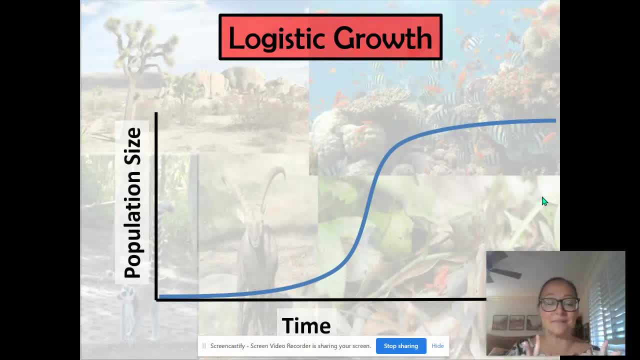 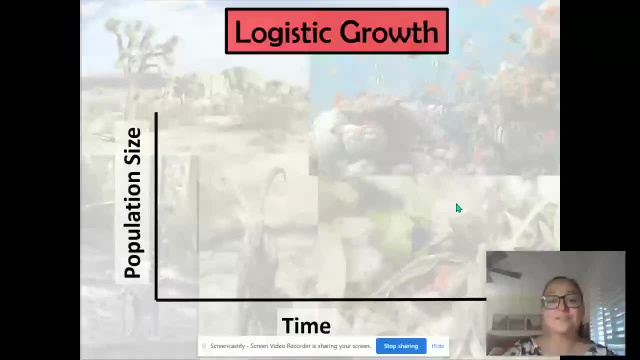 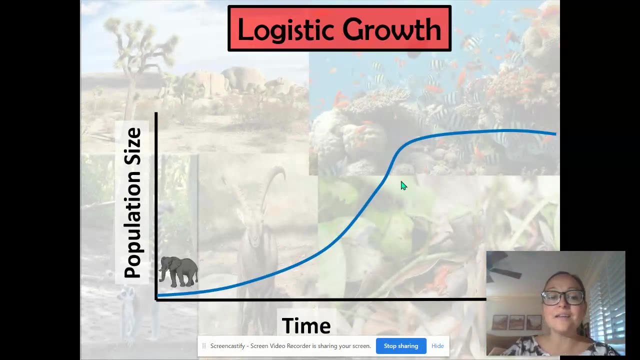 but eventually competition predators, disease, limited space, limited water, limited shelter, et cetera will limit how big a population can grow, will limit how big a population can grow. And so when we look at this logistic growth where the line plateaus, or that straight flat line, 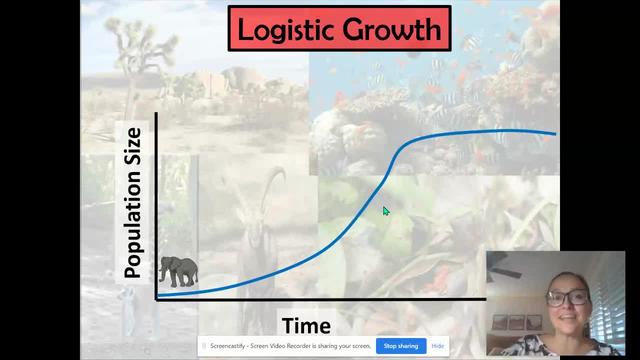 oh, just kidding. let's use the example of some elephants. So in the early 1900s, elephants were almost hunted to extinction for their ivory tusks, And then, once the different governments in Africa put a mechanism in place to shape these, Mazat сбац. 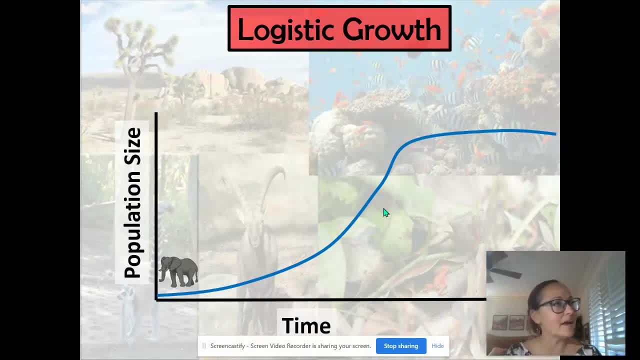 limits. I don't know if these numbers are from Kenya- I forget the country in Africa where I got this from- But let's pretend that they banned hunting from elephants and the elephant population began to rebound- And it really did happen. I just can't remember where right now. 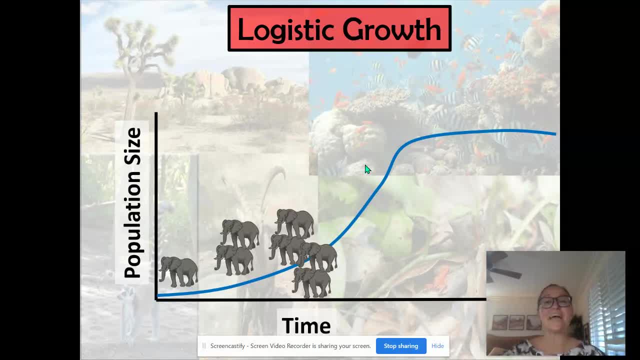 So here, initially, all of a sudden, there's protections on elephants. The numbers got so low that when you remove poachers and hunters, now there's unlimited space, There's unlimited resources, There's not a lot of competition. The elephant population is going to grow exponentially. 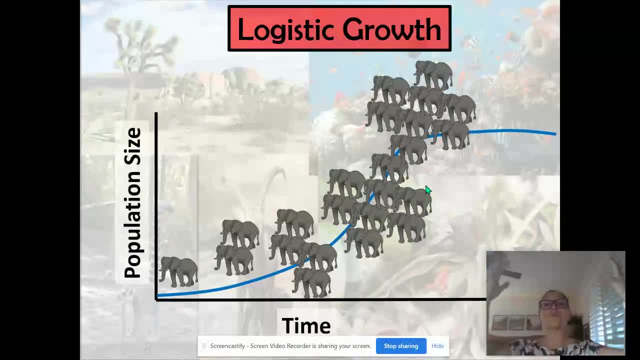 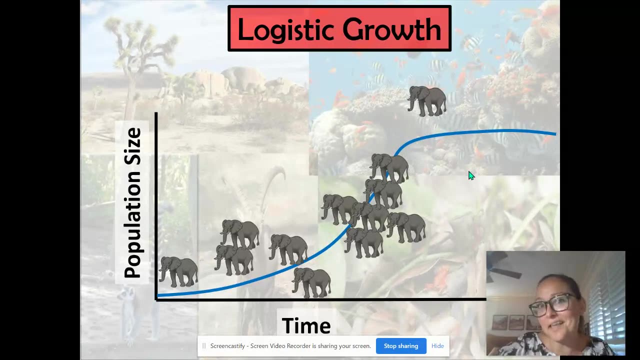 until the number gets so great, The population is so large. Now there's competition, Now there's not enough resources And you will have some of the individuals not survive And then the population size will shrink. Well, now there's less, So hey, there's a little bit more can survive. Oh no, Now we're back to 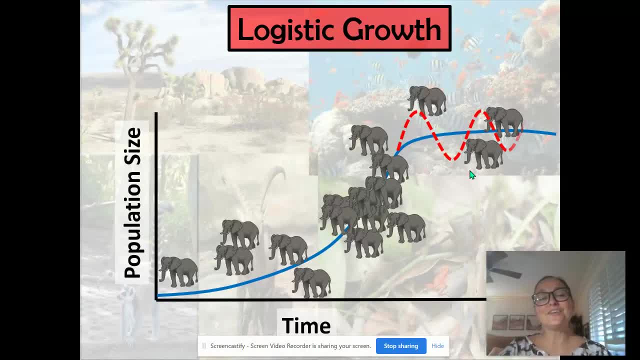 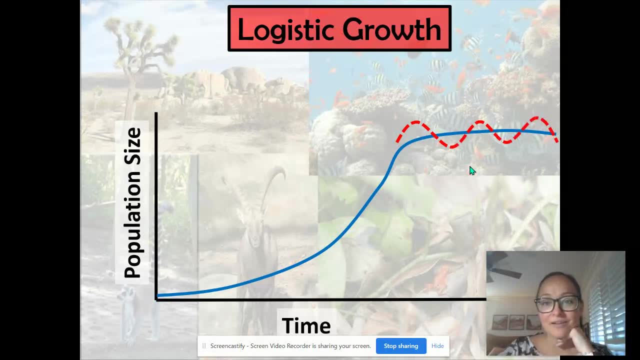 too many And then a few will die And eventually you get this fluctuation. Now, if we find the average of this, we call this area right here on the graph, the carrying capacity. So the carrying capacity it's an amount or a number And it represents the maximum number of individuals. 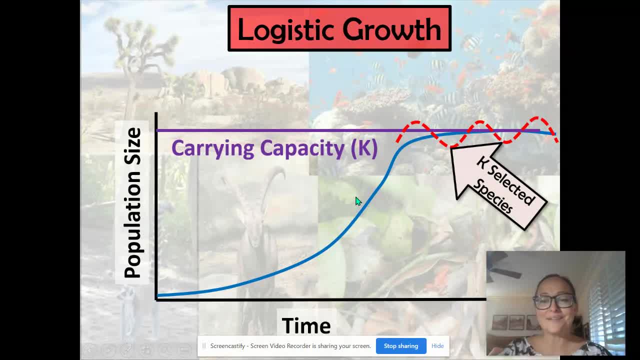 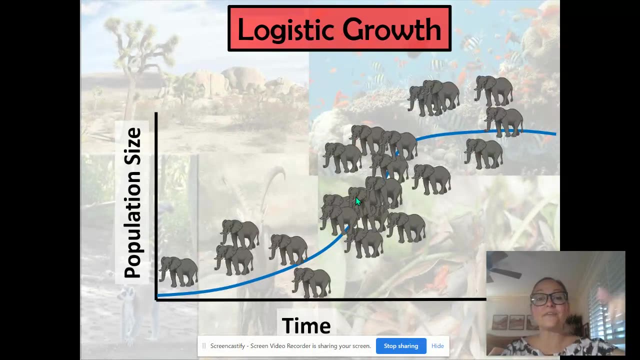 that an environment can supply. I don't think I have it defined on my PowerPoint, So let me say that one more time. The carrying capacity is the maximum number of individuals that an environment can support. So if we go back to this elephant here, it's above carrying capacity. There's too many, So then a few die, And so if we